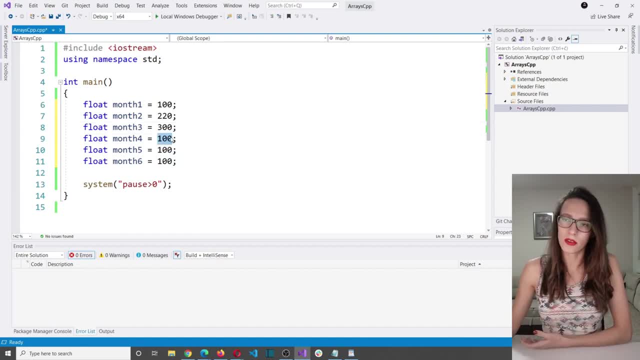 example. And then in the fourth month we had a birthday or we bought something very expensive, so we didn't save any money in the fourth month. And then let's say, $200 and $250.. Okay, so here we have stored the data about how much money we have saved each month for six months Now. 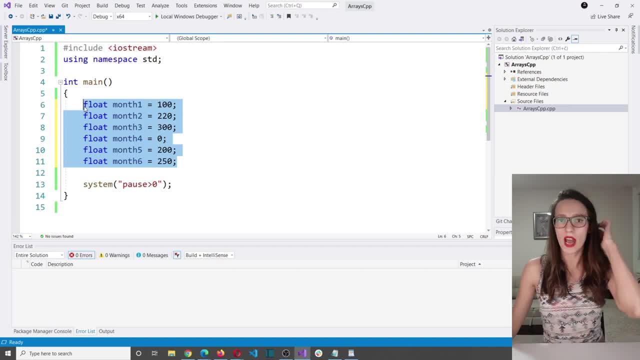 the things that I want to calculate from this data here are going to be how much money we have saved in total- So let's write that here, So total- and then how much money we on average like this: Oh, it's not average, It's average, Okay. So, and then I also want to check. 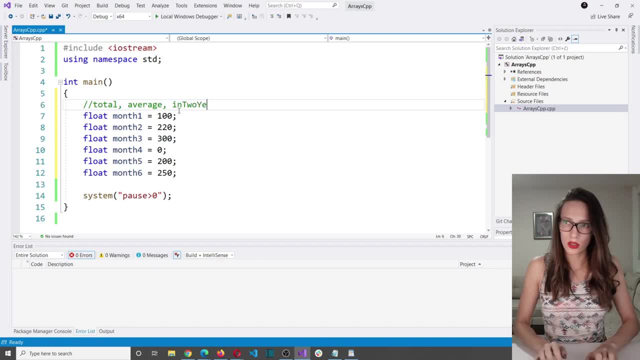 how much money I will have in two years. Okay, Now how do we calculate these three things from this data here? Well, it's going to be pretty simple. We create another variable which we will call total, And our total will be sum of these. 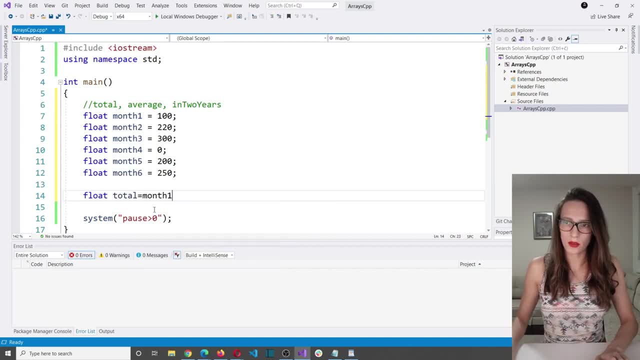 Six variables, So month one plus month two plus month three. Okay, So I have skipped this part of the video because it is pretty simple. So you just sum all of these values in these six variables And that is going to be total amount of money that we have saved in six months Now. 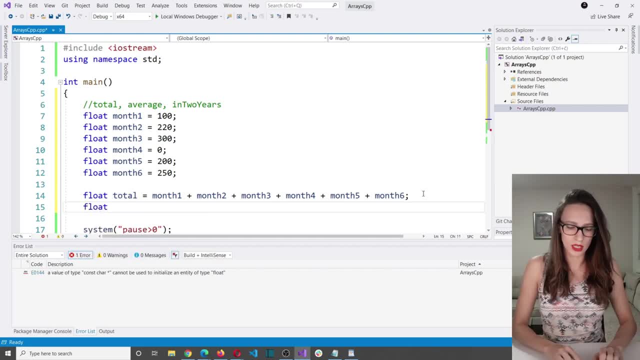 average is going to be as well of type float And let's call that variable average, And it is going to be divided by six, like this: So how much money we have saved in six months, And we are going to divide that by six months And that is going to give us the average. Now, how do we predict? how? 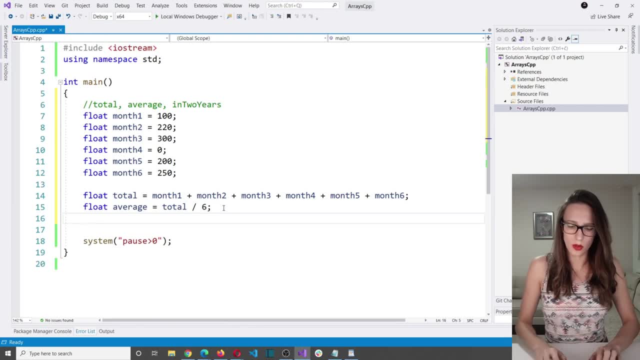 much money we will have in two years. Well, let's create another variable of type float again, And let's call it in two years, And here it will be average multiplied by 24.. Why? Because two years have 24 months. Okay, Great. Now I will write this data out to our 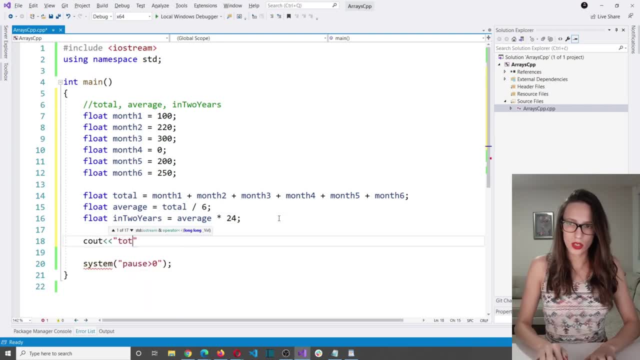 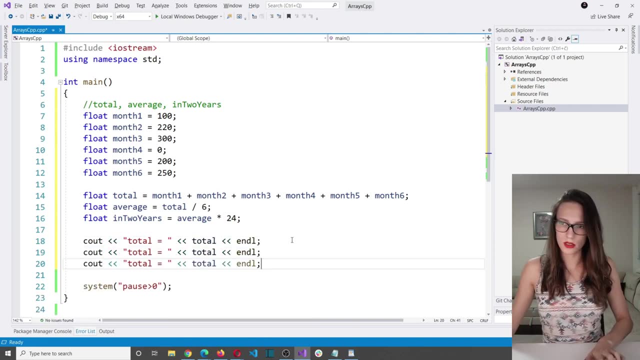 user. So let's say: cout total is equal to, and then total like this, And let's copy this three times, And here I want to write out average like this: And then I want to write out how much money in two years- Okay, Great, Now let's run our program. 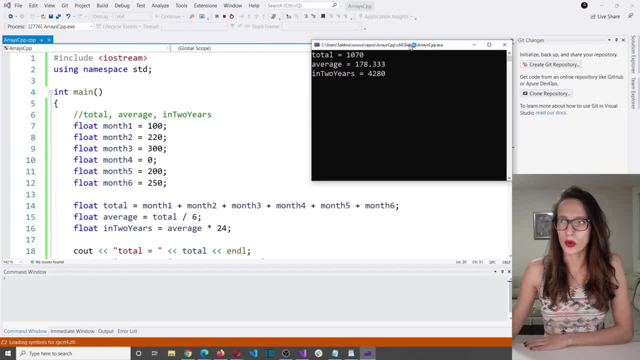 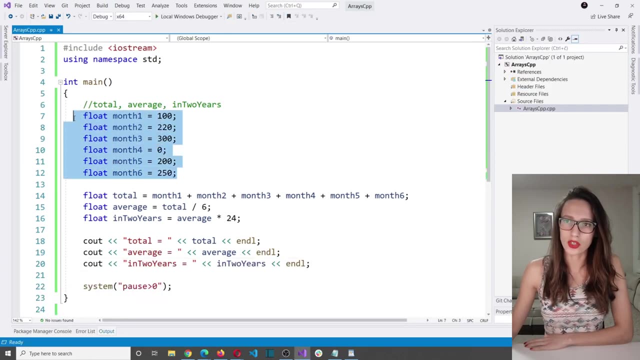 Okay. So it says: in total we have saved $1,070.. On average, that's $178.. And then in two years we will have a little over $4,000.. Okay, Great. Now this approach here works as it should. But 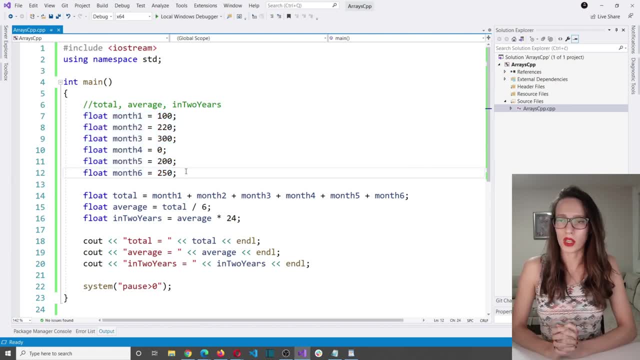 it has one problem Now. what is that problem? Well, it is pretty easy to do this when you are calculating something for six months or seven or ten. But if you are calculating something for- imagine if you had to do this for 100 months or 1,000 months- you would have to create a variable. 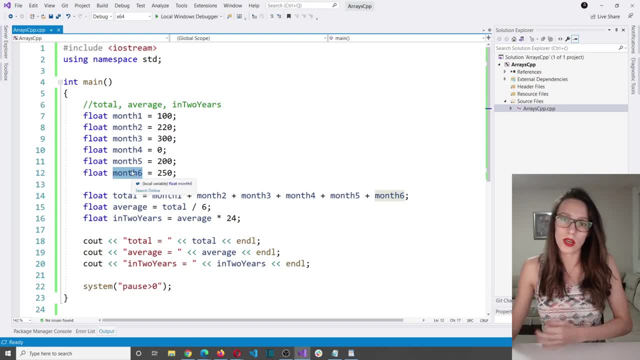 for 100 months. So 100 variables or 1,000 variables, And that is a problem. So because of that, we have a special type of collection which is called array, And we can use that collection which can group all of these variables on a single place. Now, how do we create arrays? 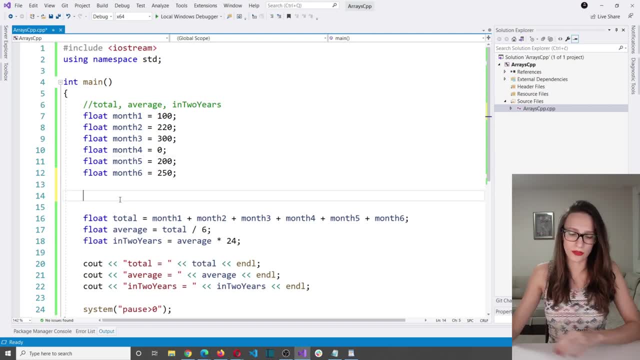 The way to create an array is following. First, you specify the type of that array, like this: Okay, The type of our array will be float. Why float? Because in that array we want to store these variables here And as you. 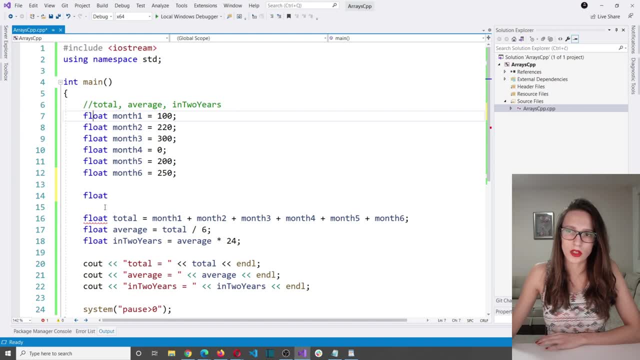 can see, all of these variables have the type float. So this is going to be the type of our array. And then the second thing is you specify the name for your array. Now, considering that our array will save the values that previously were in these variables, here, let's call that: 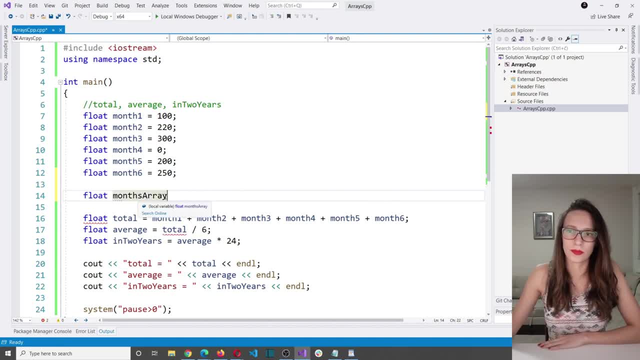 array, months array like this, Okay, And then one more thing that you have to specify is the size of that array, And how do you specify the size? You specify the size in these square brackets, And, considering that this array here will store these six values, it is going to be array of six. 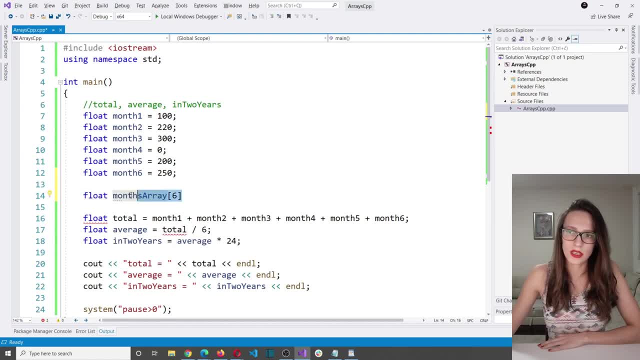 elements like this. And with this here we have successfully created an array which is called array. It can store six elements, and those elements will be of type float. Now, how do we assign values to these six elements? Well, you use these curly brackets and inside these curly, 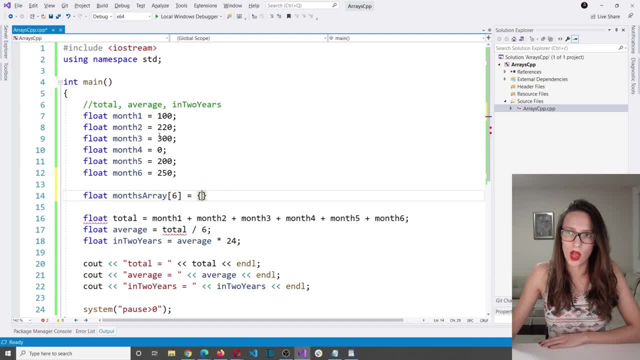 brackets you assign the values for these six elements. So I will just use these values here. So the first element will have value of 100, and then 220 and 300 and 0 and 200 and 250.. I hope. 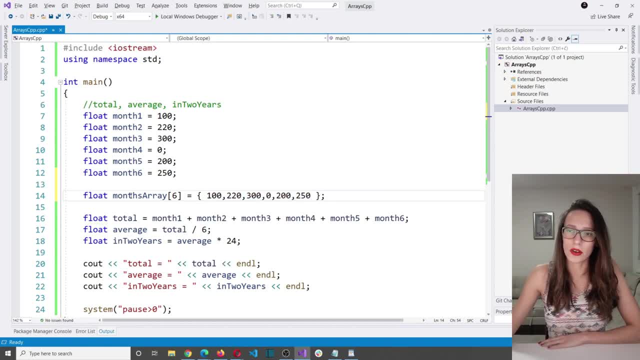 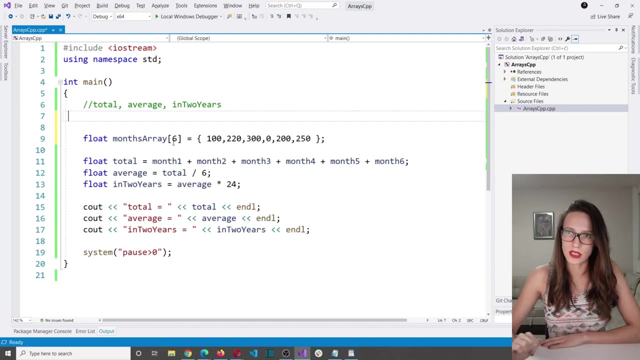 you like a mistake? Okay, So here inside our months array, we have stored these values, which are the values that previously were in these six variables. Now, that means that we do not need these six variables anymore. We can delete this part of the code here. Great, And then, as you can, 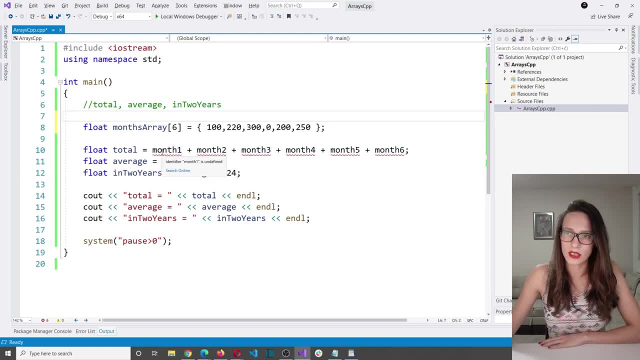 see we get an error here. It says now that month one is undefined Identifier: month one is undefined. And then it gives us the same message For month two, and then month three, four, five and six. All of these are now undefined. Why? 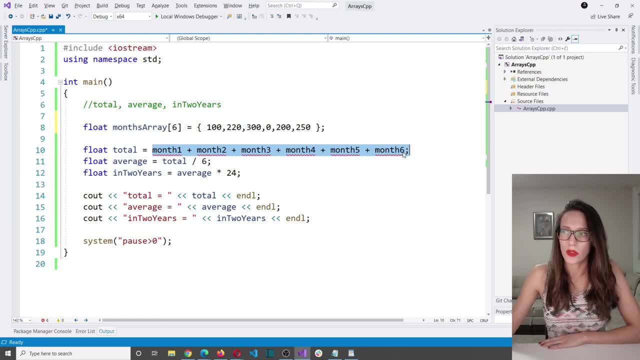 Because we have just deleted the variables that we had here. So now what I have to do is I have to change this variable with the first element of our array, and then this variable with the second element, and then this with the third, and so on, So that means that we can access these elements. 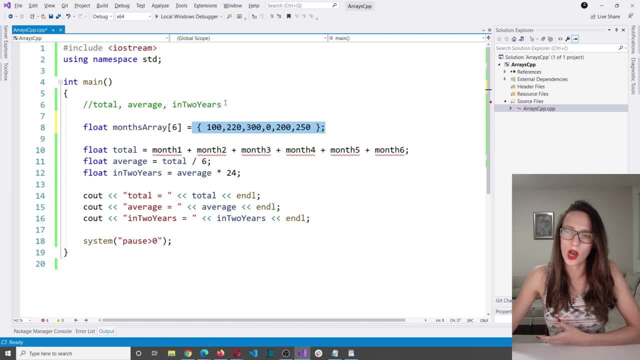 of the array individually. And how do we do that? How can I access the element, For example this element of the array? Well, in order to access elements of the array, you use name of that array and then you use index of the specific element that you want to access. 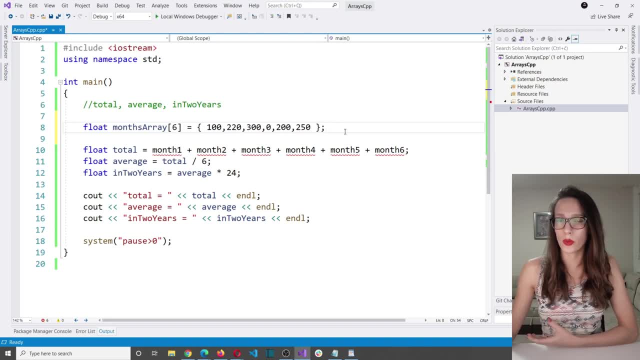 So now your question might be: how does the indexing of the array work? Well, the indexing of the array starts with zero. That means that the first element of the array has the index of zero, And then the second element has the index of one, And then third. 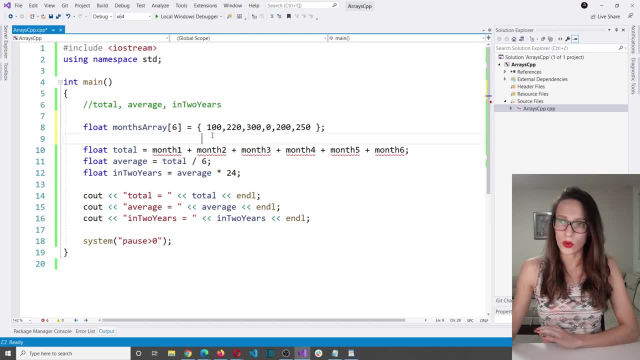 and fourth and so on. So let's write that so that we don't forget it. So the first element has the index of zero, as I said, And then second has the index of one, and then two and three and four and five. Okay, Now this here means that the array that has six elements, the indexes of those, 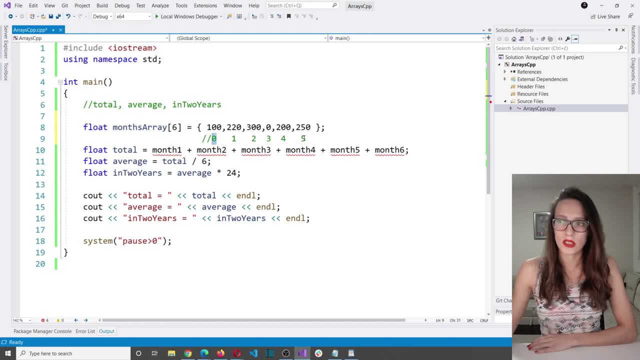 arrays of that array will go from zero to five. And then if you have array with which you know has, for example, 10 elements, the indexes of that array would go from zero to nine. If you had array that has 100 elements, indexes of that array would go from zero to 99, and so on. Okay Again. 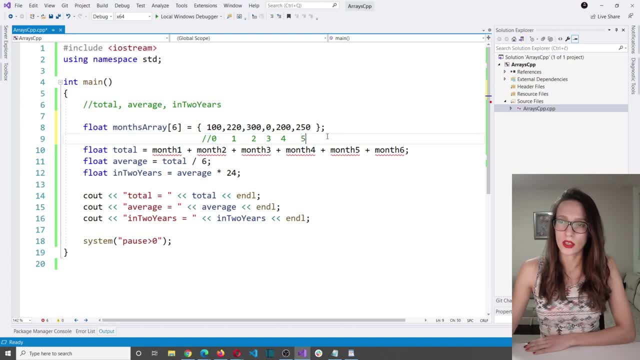 so indexing of the array starts with zero Great. So, as I said, in order to access a specific element of the array, you use name of that array and then index of that element. So that means that here, instead of this month, one variable which we previously 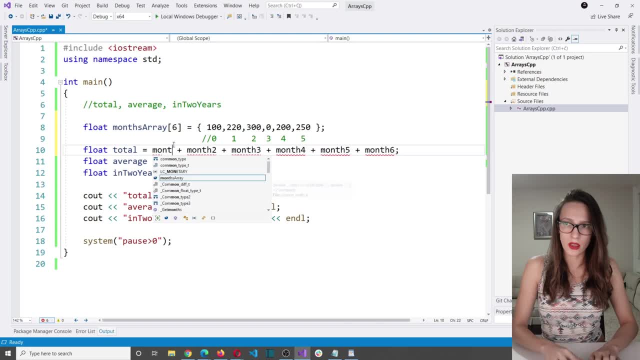 had. we will be using the name of our array, month's array, And then in these square brackets I will use the index of my first element, which is zero. So this here will give us this value here, Okay, And then here I will just copy the name of my array and then I will use index one in order. 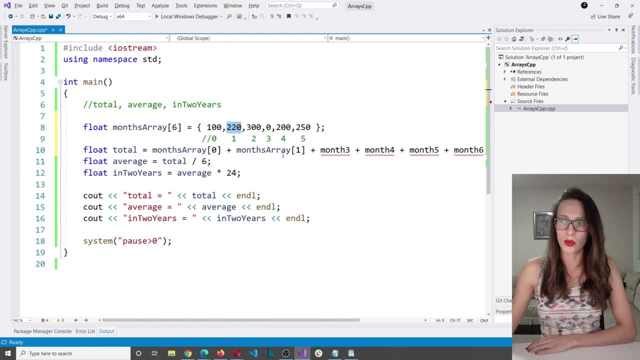 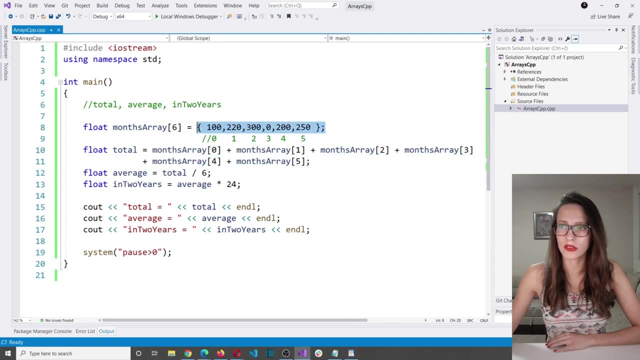 to access second element of the array, And I will do this for the second element of the array, For these remaining elements, and I will be back. So here I have total sum of all of these elements of the array, from the one with index zero until the one with index five, So six elements. 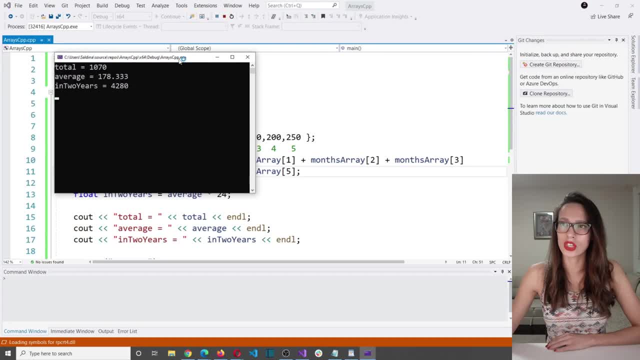 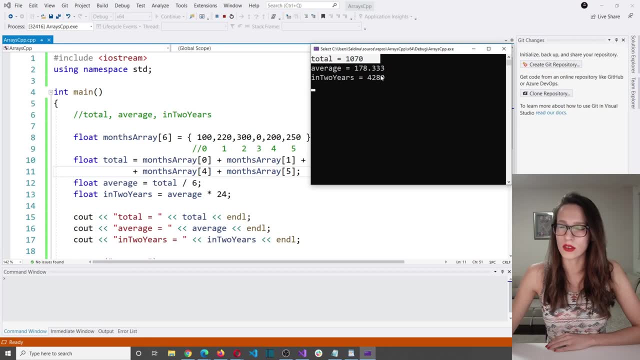 in total, And if I run my program, nothing should change. Okay, As you can see, total is again $1,070 and then average is $178.. And then in two years we will have $40 to $80.. Okay. 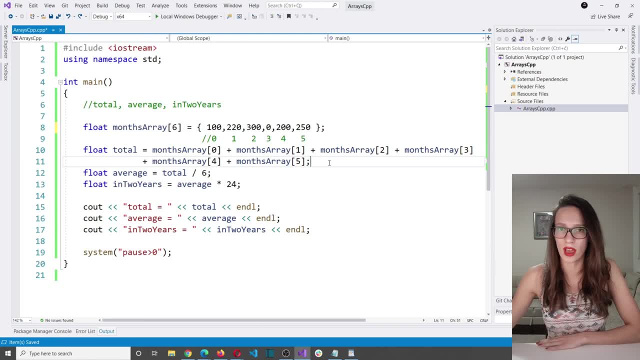 Now there is one question that I want to answer that many of you have asked, especially those that are coming from JavaScript world and learning C++ for the first time, And that question is following. Someone had asked: can you, inside this array, have elements of different types? So, for example: 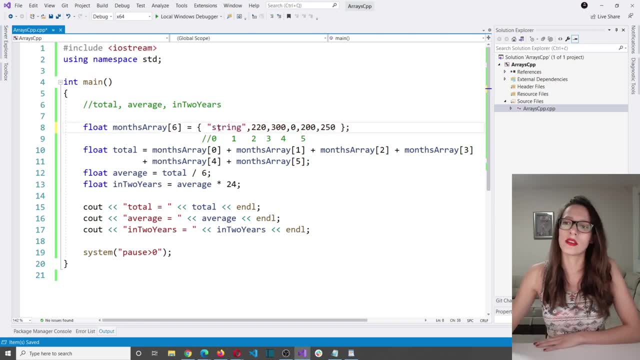 can this here be a string? And the answer to your question is: a value of type const. char pointer cannot be used to initialize an endpoint, So if I run my program, nothing should change. So here I have, total sum of all of these elements. 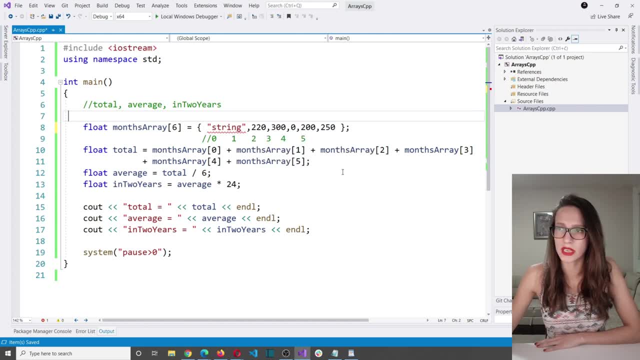 of type float. What this message here means is that, no, you cannot do this. If you created an array of type float, all of the elements of that array have to be of type float, at least in C++. In some other languages that is not the case, But in C++ all of these elements have to be of type float, or. 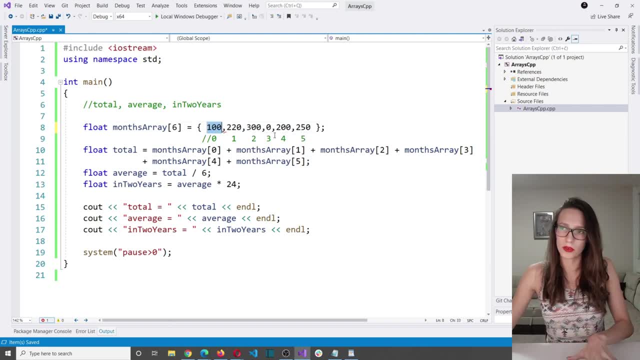 something that can be converted to float. So I will return this to 100.. And, as you can see here, this is integer. So I'm going to return this to 100.. And, as you can see here, this is integer. 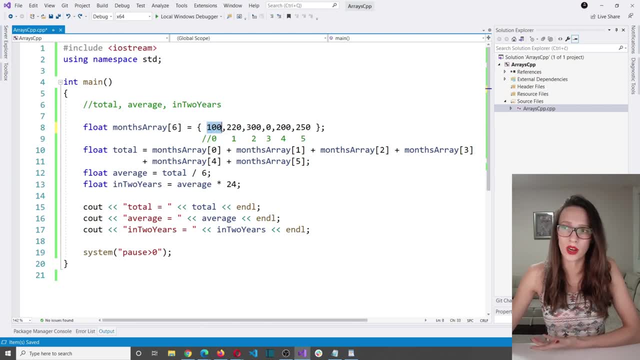 But that integer can easily be converted to float, because 100 is the same as 100.0. And this here is a floating point number. This here is float type, But it is just easier to write it this way. So the answer to your question is no. All of these elements here have to be of the type that your 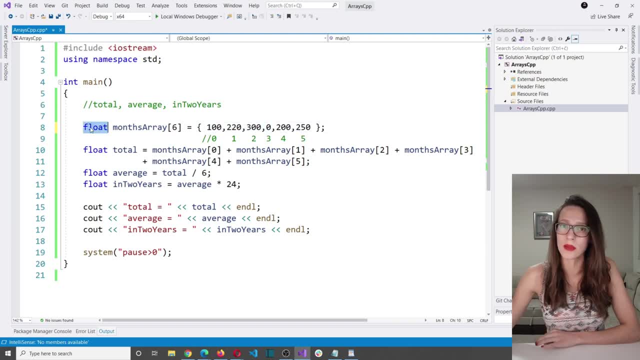 array has, So all of these elements have to be of type float or something that can be converted to float. Okay, So now that I have cleared that, let's return to this part here. Here we have learned how to access a specific element of the. 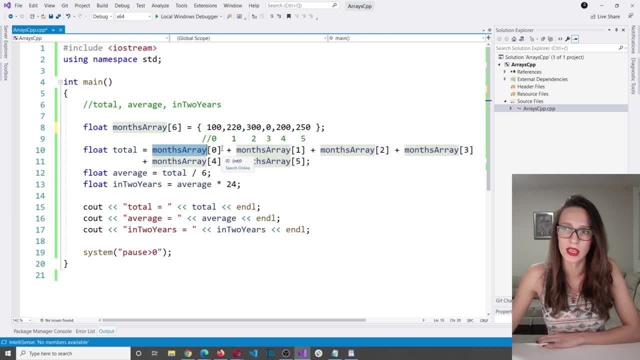 array. So you do that by using the name of the array and then the index of that specific element, And indexing of the array starts with zero. Now one more question that you might have, then, is the following: Is this part here necessary Meaning? do you have to initialize all of the 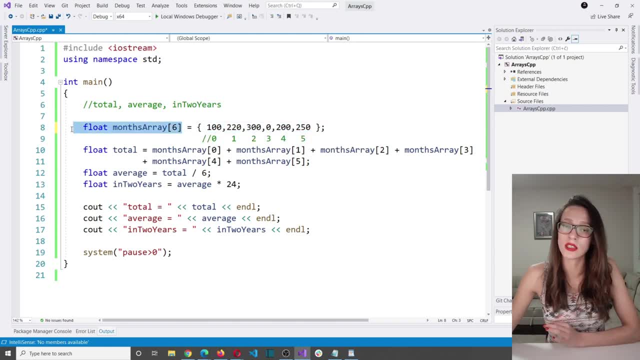 elements of your array when you create that array. And the answer to your question is no, you don't. So what I can do here as well, is I can say that this part of the code does not exist anymore. You can comment it out. You can delete it if you want. I will comment it out for 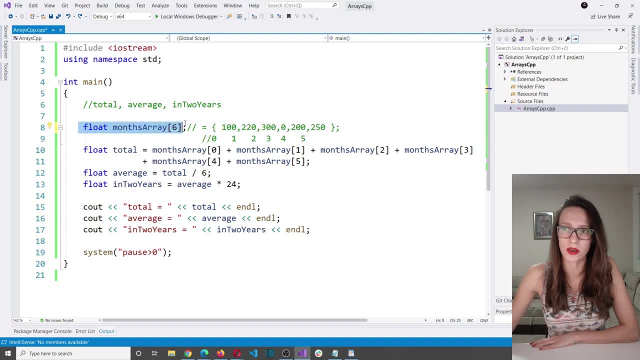 now. But what you can do basically is you can just create an array of type float that has six elements, But you don't have to initialize those elements when you create the array. You can initialize those elements later in your program. So what you can do here is you can do the same. 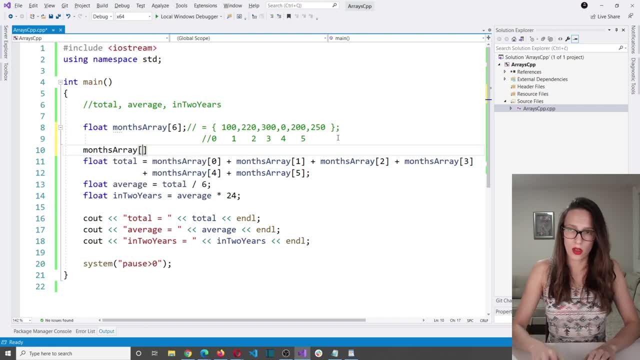 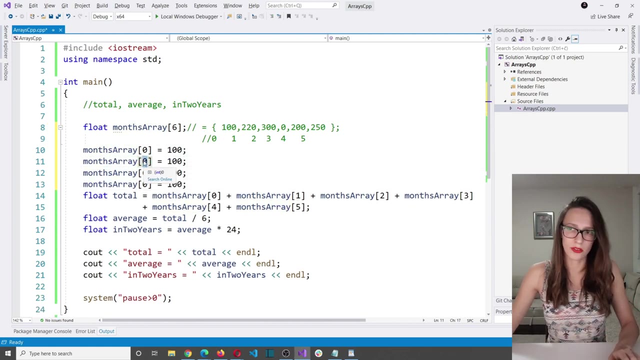 thing. You can do the following: You can say: months array of index zero. So it is our first month We'll have the value of 100. So it is this value here And then let's do. okay, let's do for. 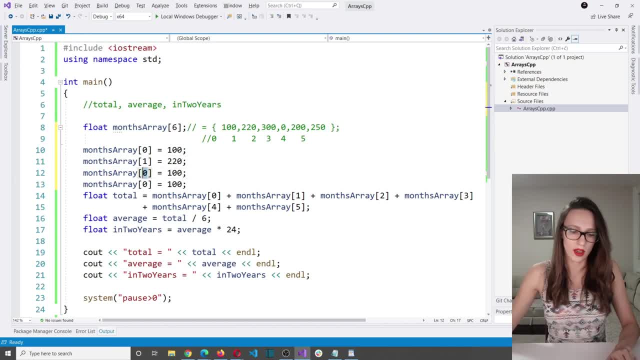 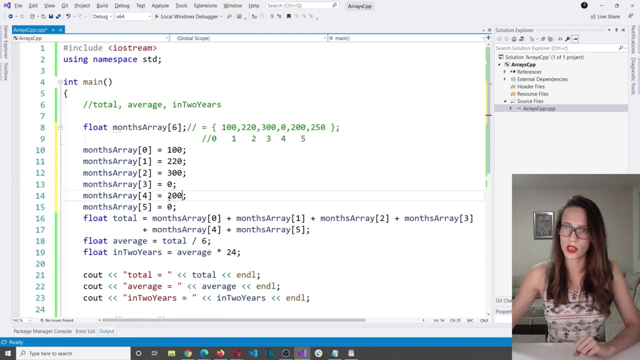 the first month, it has the value of 220.. And then our third month, the one with index two, has the value of 300. And then fourth has the value of zero. Okay, let's do two more Four and five, And these have values of 200 and 250, like this. So this here is: 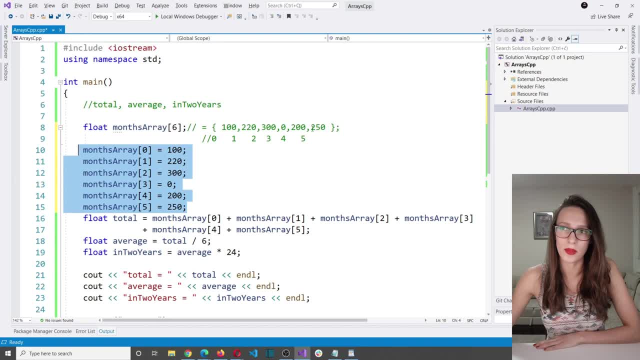 another way to initialize the elements of your array, And this is one way that we previously showed. And then this here is another way to do that same thing. So if I run my program, nothing should change, basically. Okay, So again here we have the same values that we previously. 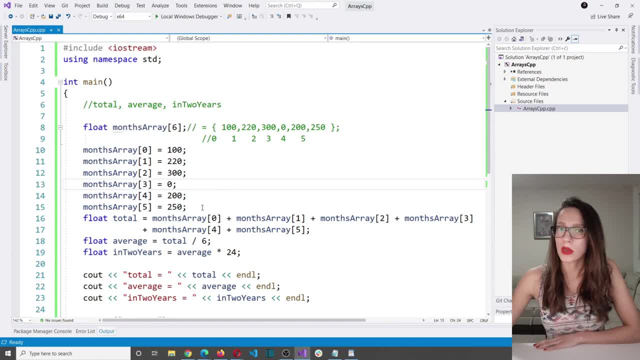 had. Okay, Now one thing that you may wonder as well is: now these values are hard coded. So throughout this program we had all of these values hard coded. But what if we want our user to enter all of these values? Well, you can do that as well. What I can do is I can say: 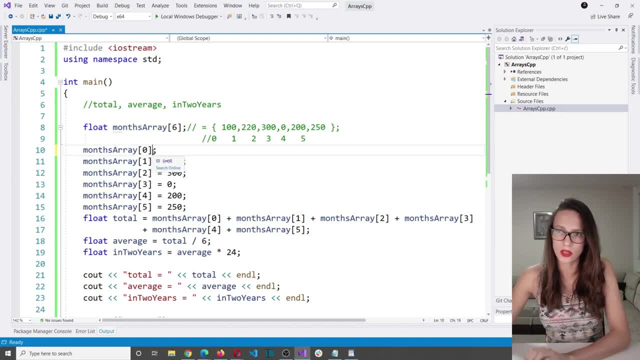 the following. So, instead of assigning this value of 100 to my first element of the array, what I can do is I can say: see in and then assign that value that our user entered to the first element of that array. So our user will input the value in our console And that 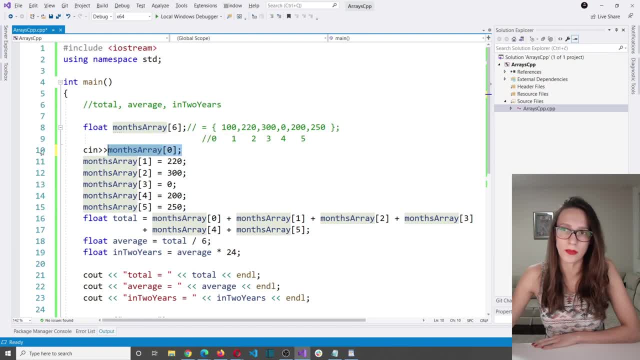 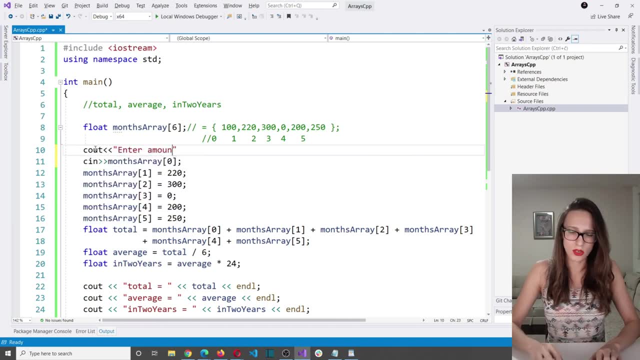 value will be stored in the first element of our array, And let's write out a message to our user as well. So let's say enter amount like this: Okay, And let's do that same thing for these remaining five elements. So let's delete these hard coded values, Okay. 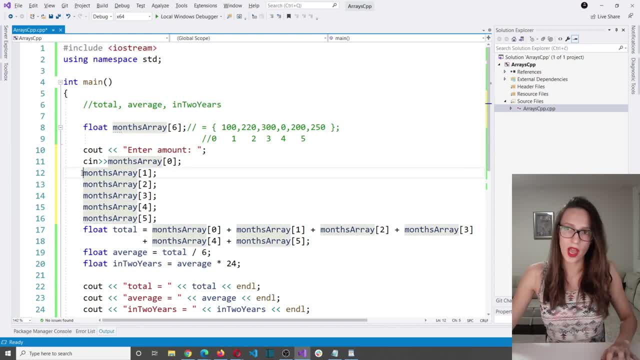 Like this, And here I want to let my user to enter these values. Okay, And if you're wondering about the shortcut that I just used to write in multiple lines at the same time, I believe it's alt plus shift. However, my brain does not know shortcuts. My fingers do. Okay, So here we have. 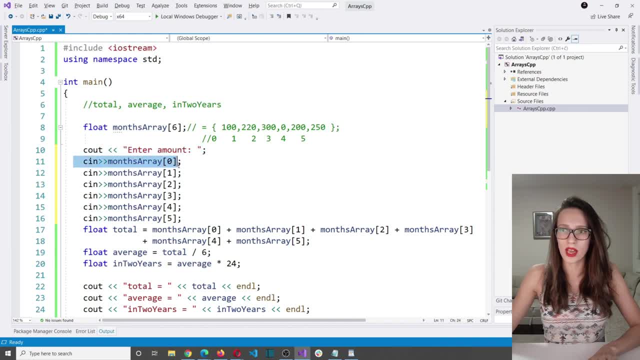 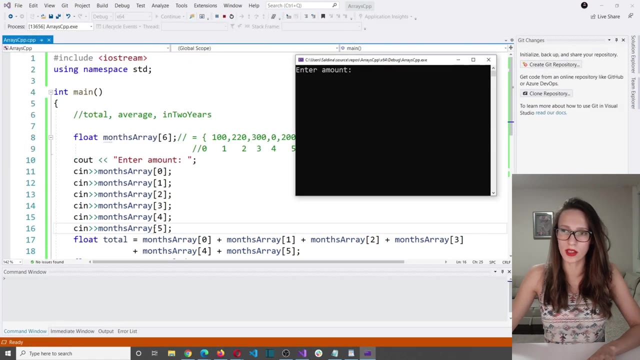 asked our user to enter amount, And then here we have entered amounts for six months in the elements of this month's array. Okay, So if I run my program now, it says enter amount And then it will store six values in these six elements of our month's array. So let's enter six values. 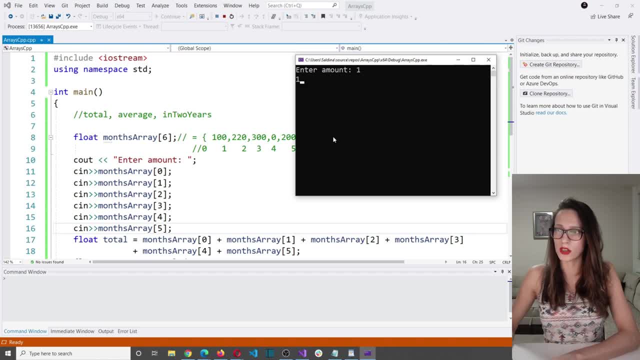 Let's say that in the first month we have saved $1, and then $1 and $1, and then $2, and then one and one again. Okay, So it says that in six months we have saved $7 and that is $1. 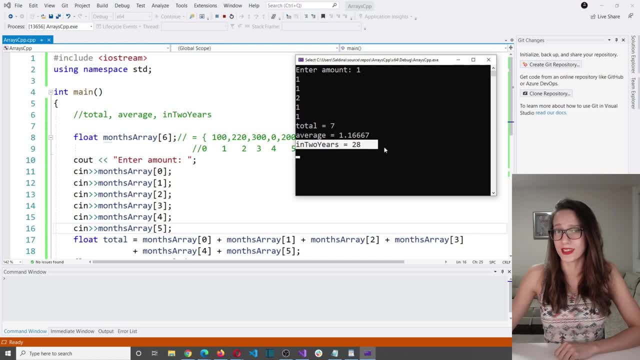 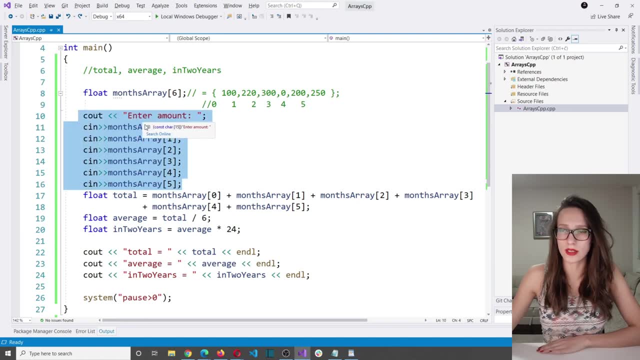 $1 a month, And then in two years, we will have $28.. Okay, Great. So, as you could see, this code here works. But I still have a problem with this code, And the problem is that it is not. 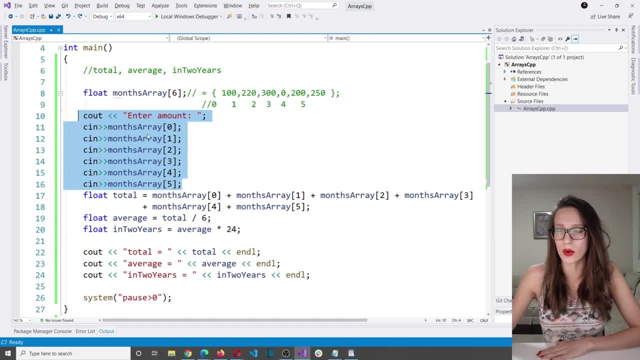 optimal. There are more optimal ways to write this code here. So it is pretty easy to do this for six elements, But if you had 12 or 100 or 1000 elements, you would have to basically do this 100 times or 1000 times or even more, And that is not optimal. So what I want to do instead of 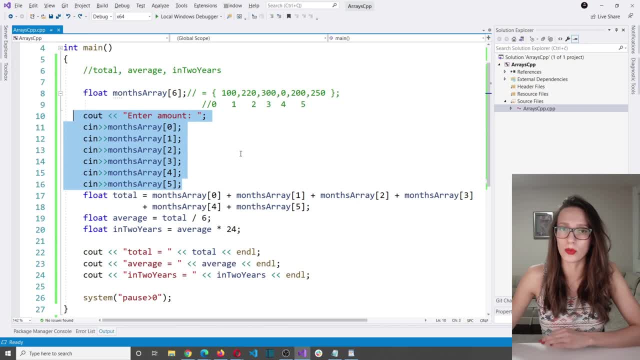 this code here is: I want to use a for loop, And if you are not familiar with for loop, I will link a video here where I explain for loop in detail. So make sure to watch that, Okay, So let's just. 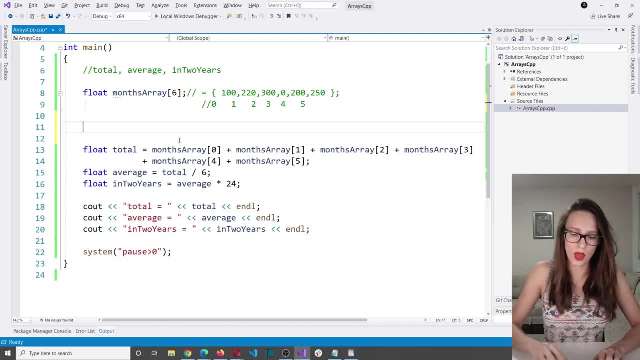 delete this part of the code here. So I will say for, and then I will create a counter of type int and give it minimum value. So I will say for, and then I will create a counter of type int and give it minimum value. 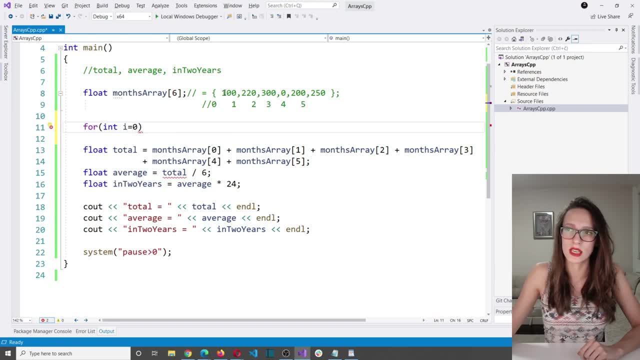 of 0. And you should notice that the first element of our array has the index of 0. That's why we are starting this counter with the value of 0. And then we will say that that counter will have the maximum amount of 5.. So, while i is less than 6, you could do as well while i is less than or equal. 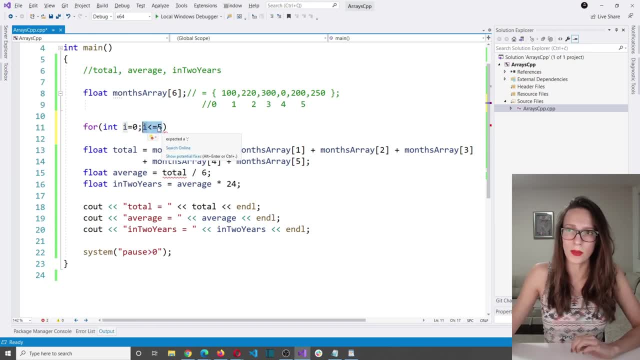 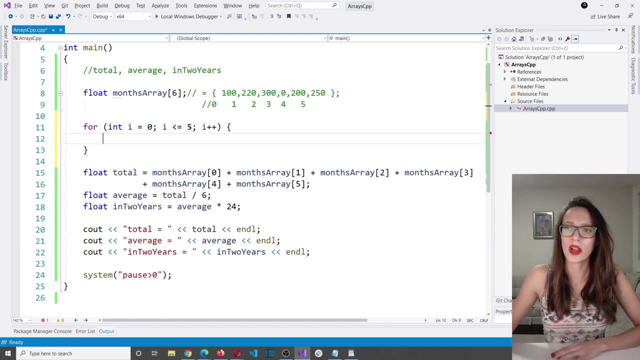 to 5.. You can do it this way as well, And this number here is the maximum index of the array that has 6 elements, And then in each iteration i will increment this counter by 1. Great. So what I want to do in this for loop is: I want to say cout. 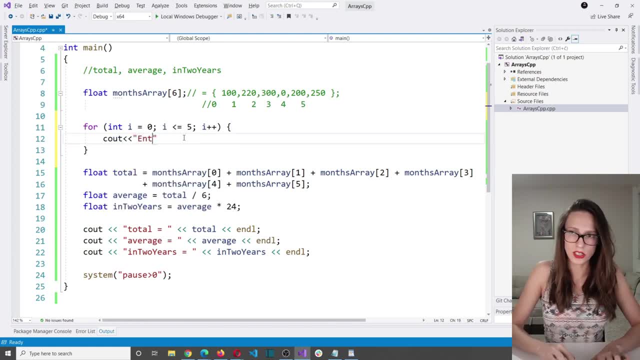 1 in this for loop is i want to say: cout- Enter amount element. and then i will write my counter. i like this. So I will say to my user: please enter the amount of the amount for the element that has this index here. and then what I want to do is I will say: 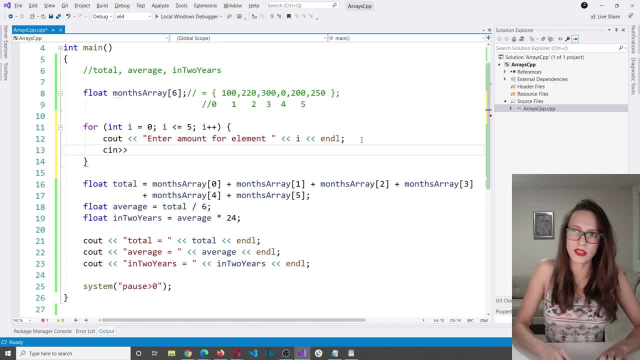 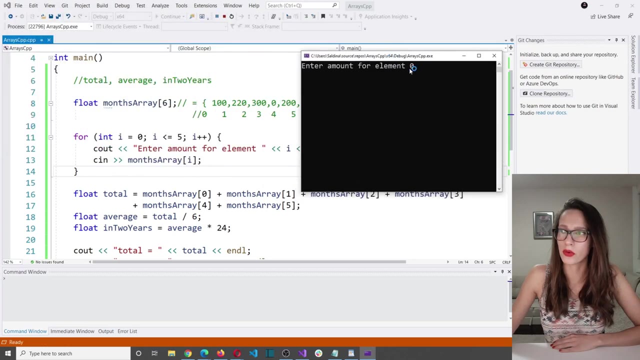 c in. okay, we use these other redirection signs c in months array, and then I want to enter the value for that specific element like this: Okay, great. Now if I run this program, it says enter amount for element zero and that amount will be, for example, one, and then it says enter amount. 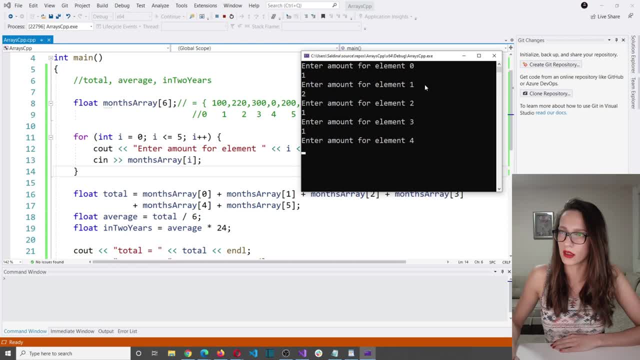 for element one, let's say two and then one again. Okay, so it says that in total it is seven, and then on average it's 1.1, and then in two years it's $28.. Great. Now one thing that I don't. 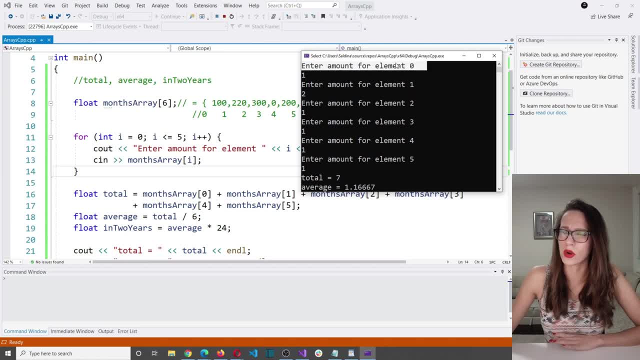 like. here is the way that this, here, this message, sounds to our user. It says: enter amount for element zero. This really does not make sense to someone who is not coming from programming world. This element zero does not make sense to your user, so it would be much. 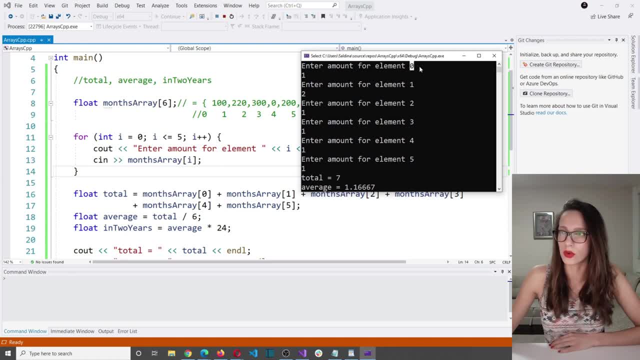 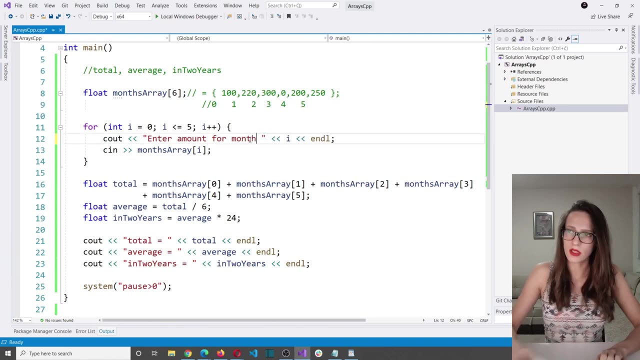 much better for this to start counting at one for your user. so it would be much better if it said: enter amount for element one or month one, for example. So I will just adjust that output and we will do that here. So instead of element I will write month, like this, and then here: 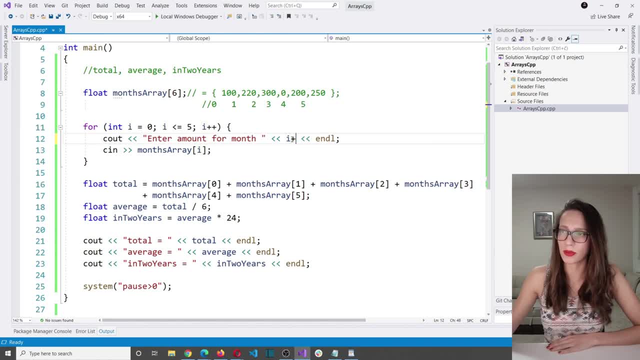 instead of I, what I want to write is: I want to write I plus one, because we do not want for our first output in the console to say enter amount for month zero because we don't want to have month zero does not make sense to anyone who is not coming from programming world. And then here, 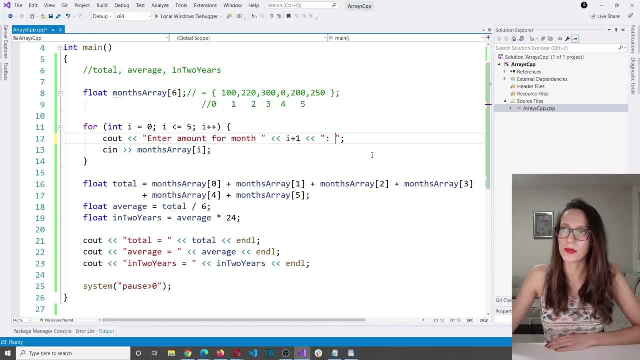 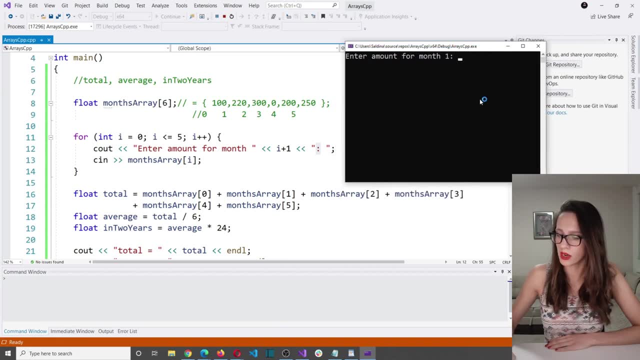 instead of this end line it would be better to add this colon sign. So if I run my program again, it should be more natural to our user to enter values. So it says: enter amount for month one. I enter one, and then two, three, four, five and six, for example. So here we have our total. 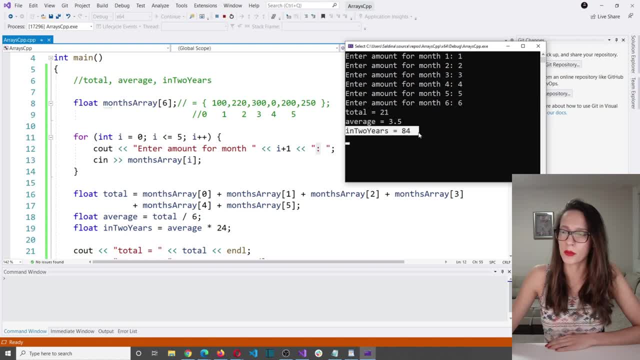 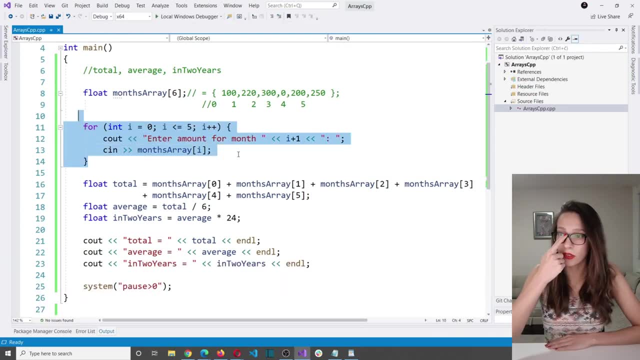 our average and then our estimate in two years how much money we will have in two years. So now this code here looks much better. But another problem that I have here is this part of the code here. So what we have achieved with this for loop is the following: We can say now: 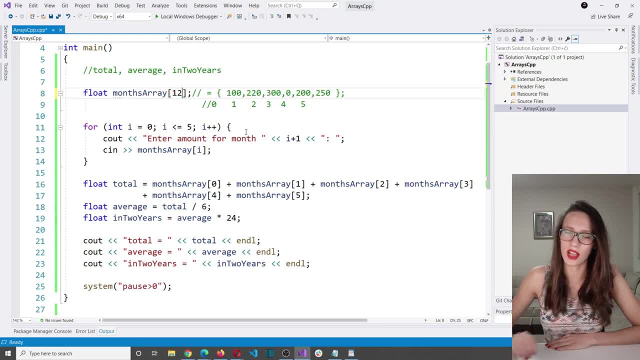 please, can you create an array that has 12 elements, for example, or 100 or 1,000 elements, And the only thing that we would have to do in this situation is adjust this index here. So indexing of the array that has 12 elements. 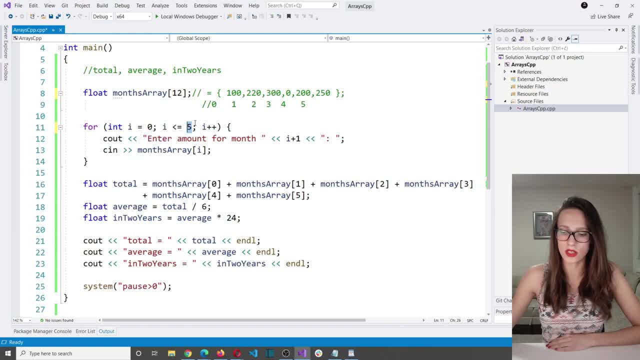 starts with zero and then the last element has the index of 11.. Okay, Now, this code here should allow us to enter values for 12 months, So from the one that has index zero until the one that has index 11.. But if we just change this part of the code here and then this part here, and we run our 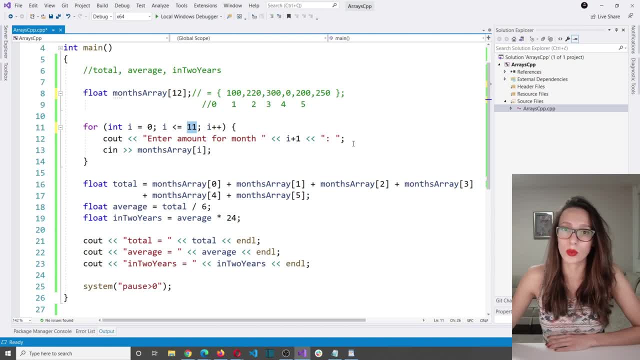 program, we will have a problem, And can you predict what kind of problem will we get? So write that in the comments down below. And the problem: without running this code, because I already know that there will be a problem with this line of the code here. If you want, you can run it and then see that all these calculations 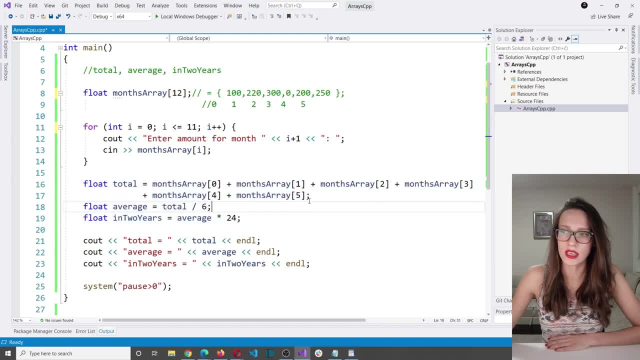 now will not be correct anymore, because here we have hard-coded six months, So here we are summing the total on six months And here we are creating an array of 12 months and entering 12 values. So these calculations here are not going to be correct. 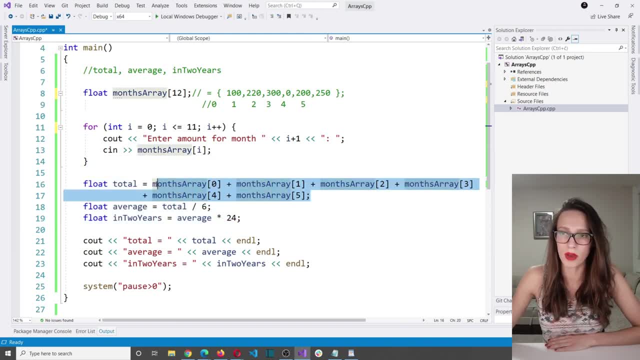 anymore. So what I want to do is I want to remove somehow this part of the code here, So I do not want to hard-code this anymore, because this is a problem as well. So how will I do that? Well, 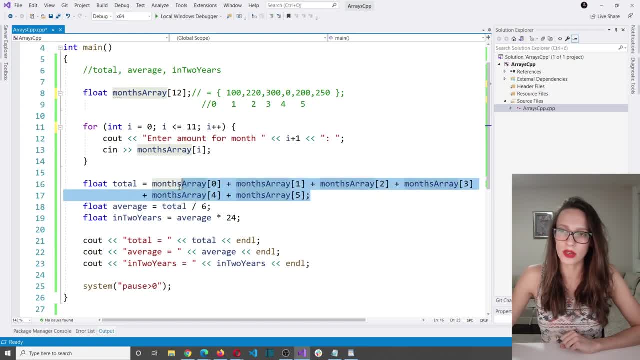 what I can do is I can move this part of the code that sums values of each month in our for loop as well. So how do we do that? Let's comment this part of the code here for a moment, And what I want to do is I want to create. 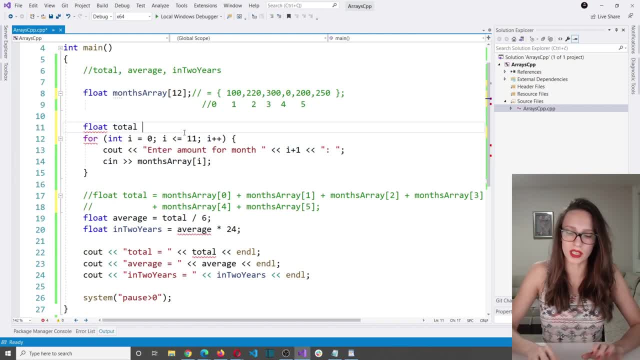 a variable of type float, which I will call total, because we definitely need a total, And to that variable I will assign a value of zero. But instead of hard-coding this part of the code here, instead of summing the values in our six months like this, what I want to do is I want to 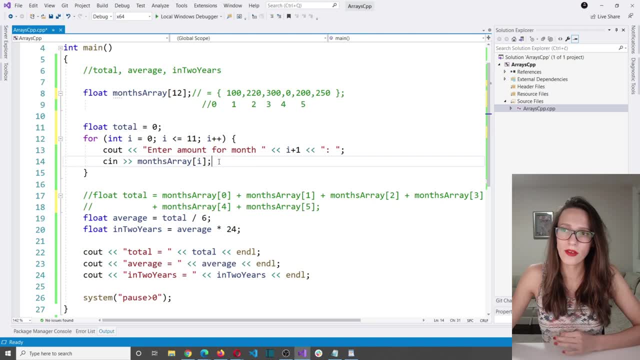 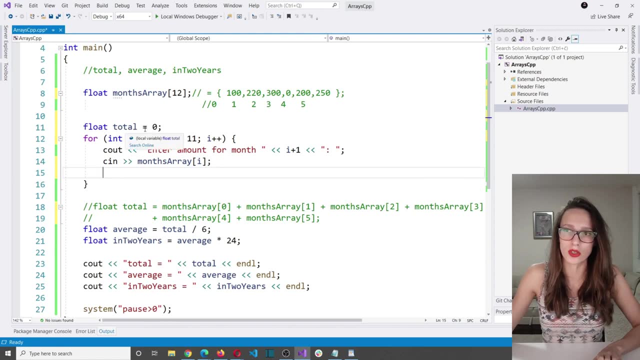 sum those values in this for loop here. So after our user enters value for that specific month, I want to add that value to my variable called total. So here I will say: total plus equals two and then month's array of: i. So 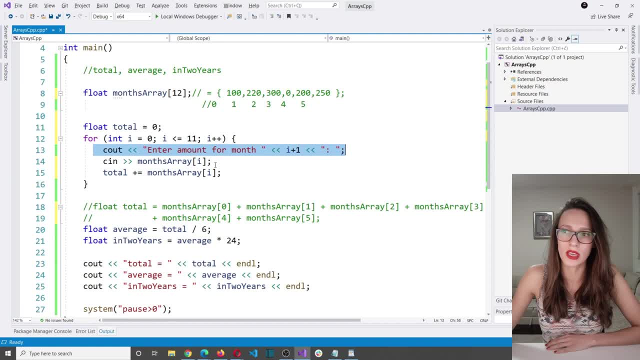 in the first iteration, when we ask our user to enter the value, he enters that value. That value is stored in this variable here. We add that value to our total. And then we go for the second iteration, And then our user enters second number. We store that number in this variable here. 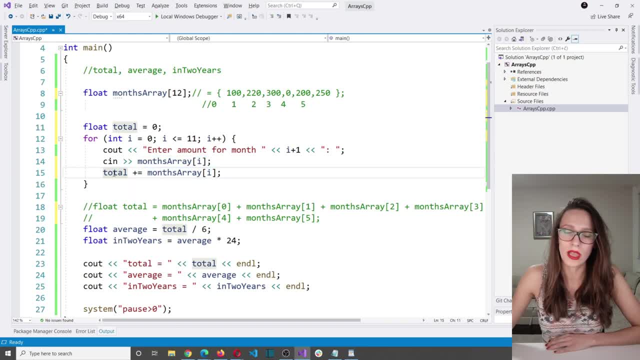 And then again we add that number to our total, And then in the third we add third number, fourth, fifth and so on. So that is why it is important for this variable here to have initial value of zero, because zero is neutral when it. 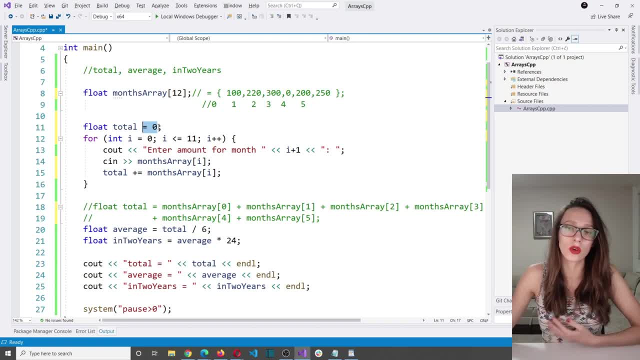 comes to operation of adding, Whatever you add to zero, it is still going to be that same value. It's not going to change. That's why we have initialized this variable here to zero. So now, after this for loop finishes, we will have the correct value in our total variable, But we still 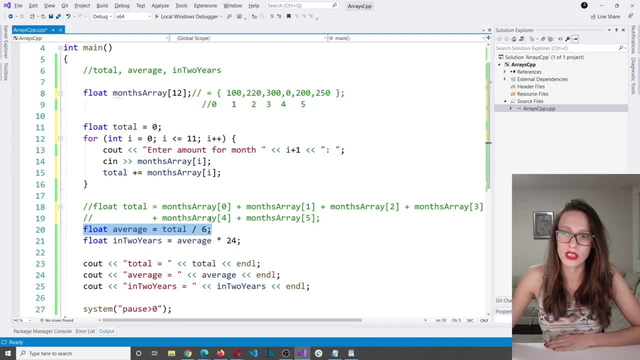 have to adjust it to six. So here it says: average is equal total divided by six. And as we change this value here from six to twelve, that means that we will not be dividing this total by six anymore, But here we will have to adjust it to twelve as well. Okay, So now, if I run my program, 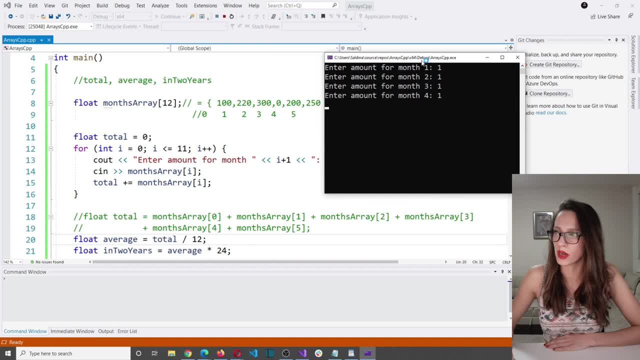 and then, if I enter, let's enter one one one, so that we can check easily. Okay, And then let's enter two as well. So now, if I run my program, and then if I enter, let's enter one one one. 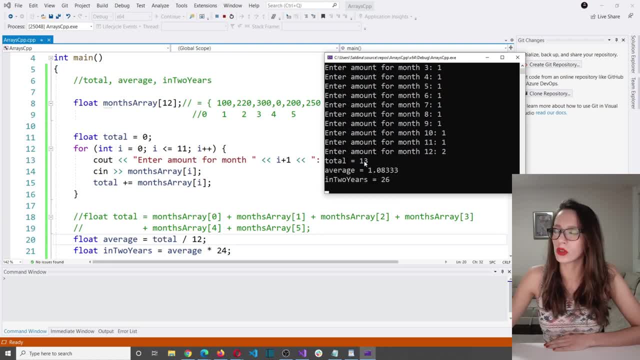 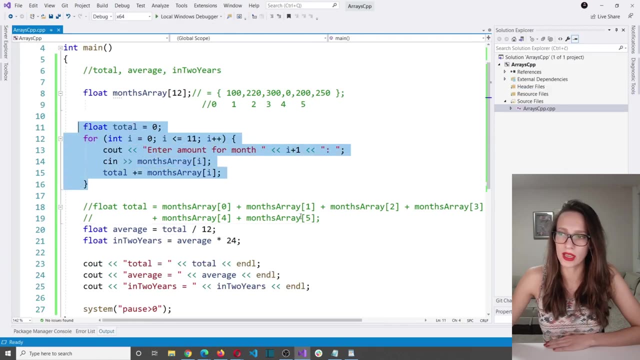 the last value, Okay. So it says: in total you have thirteen, which is correct, And then on average you are saving a little more than a dollar, And then in two years you will have twenty-six dollars. Great, So that means that this code here is working, And that means as: 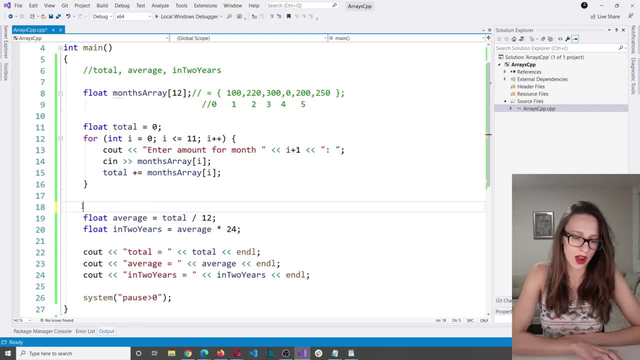 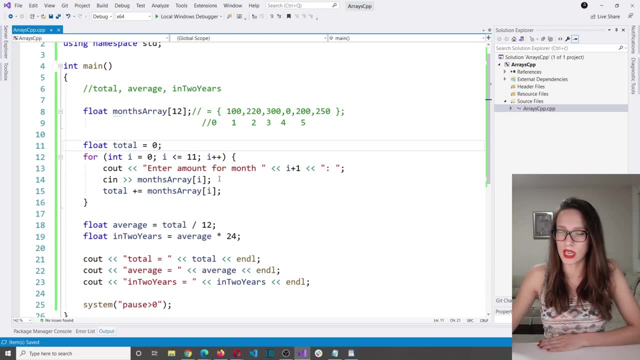 well that I can delete this part of the code here, which was hard-coded. Okay, So I hope that you understand what we have accomplished with the changes that we have made. And again, if you don't understand for loop, I will have a link in the description of this video where you 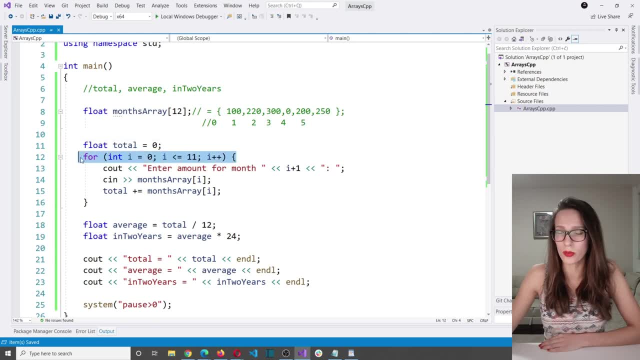 can click and watch a video which is related only to for loop, and then understand what this part of the code is doing in more detail. Okay, So again, what we have accomplished with the changes that we have made is the following: Now we can very easily adjust this value. here, For example: 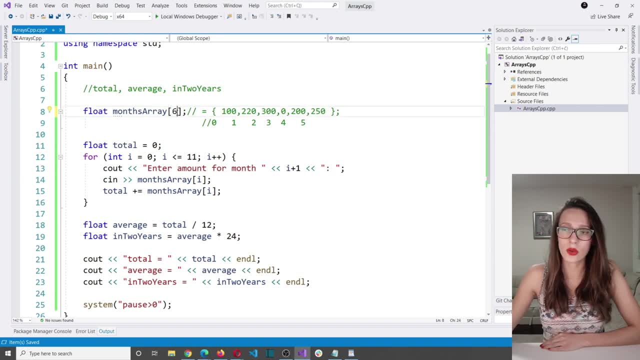 let's make this six again, And then the only things that I have to change is this index here. So the array that has six elements has indexes from zero to five. So here I will have to write five, And then here I will have to write six again. Okay, And if I run this code, let's check. 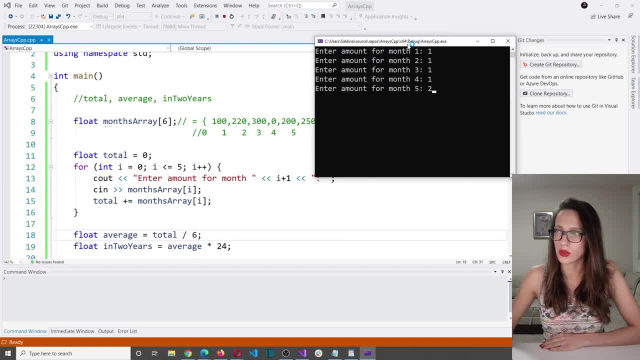 it one more time: One one, one, one, two And then six. for example: Okay, It says that total is twelve, average is two, and then in two years we will have forty-eight. There is one more. 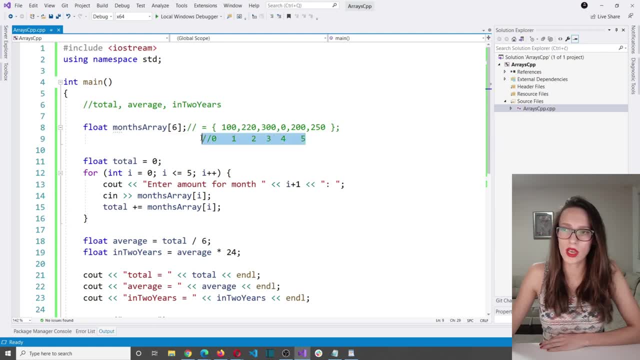 thing that I want to show you, And that is why did I say that we have to obey these indexes here, Why the array that has six elements, why it needs to have indexes from zero to five. What will happen if we put here six, for example? Well, let's try, Let's run our program, because we will. 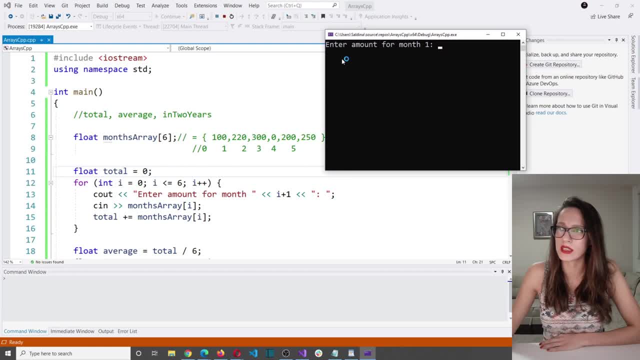 never know if we don't try So again. it says: enter amount for month one, and let's do that, Okay. And now it is asking to enter amount for month Seven, So let's enter one there, And everything works as it should, apparently, Or does it What? 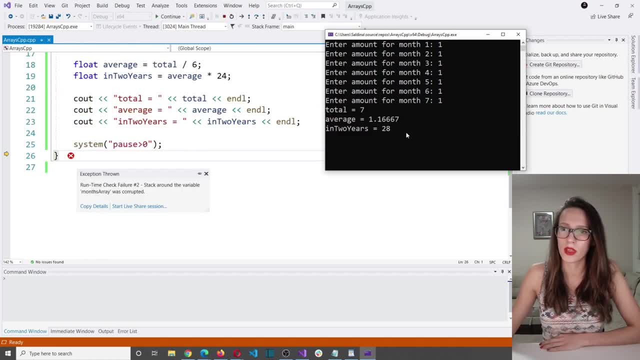 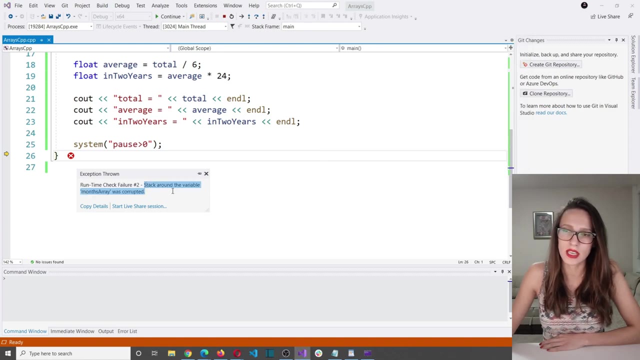 happens if I press one more time, enter, for example: Oh, so we get an exception, And that exception says runtime check failure, and then it says: stack around: the variable month's array was corrupted. Well, what this here means is basically we are using a memory which does not belong to. 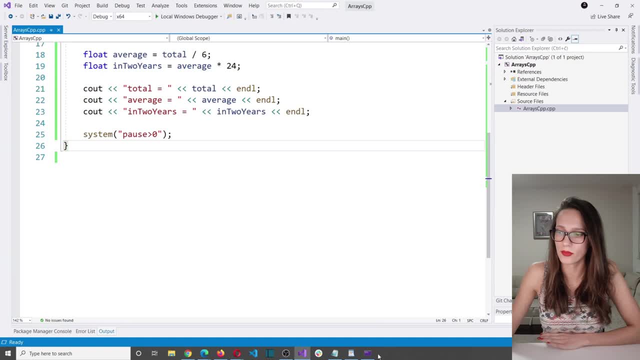 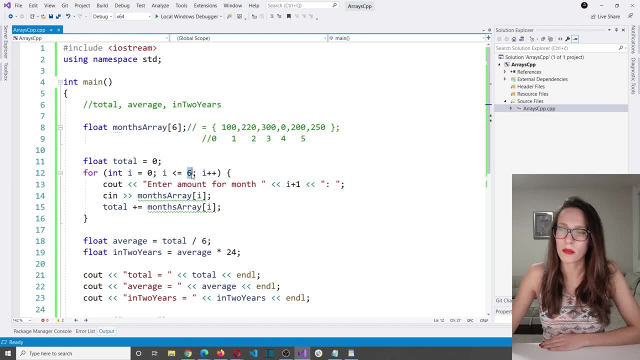 our array. So I will close this now And I want to explain this part of the code here. The indexes in this for loop go from zero to six, But the valid indexes of this array are from zero to five, which means that if we try to access the element that has index six, that element does not belong. 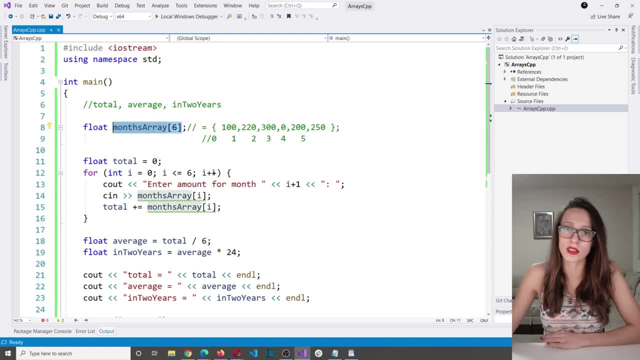 to this array here. That element is someone else's memory And if we try to do that, we can get serious problems, as you already saw. So we got an exception which said that stack around this array here was corrupted. So that means, as I said here, we have to really obey these rules. So 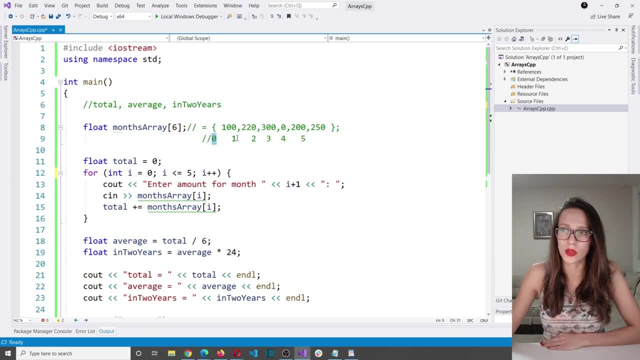 the indexing of the array starts with zero and then it goes one, two, three, four, five and so on. So the array that has six elements has indexes from zero to five. Now some of you may wonder the following: Wouldn't it be super interesting to have a set of indexes from zero to five? 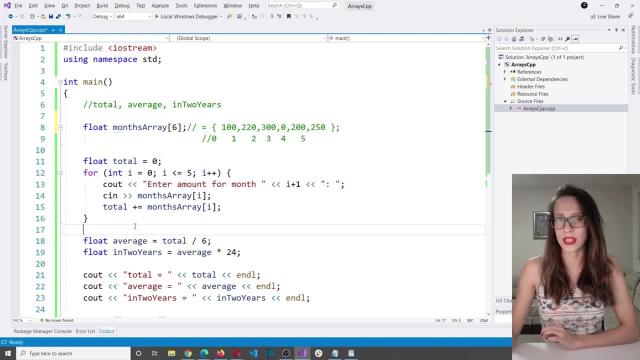 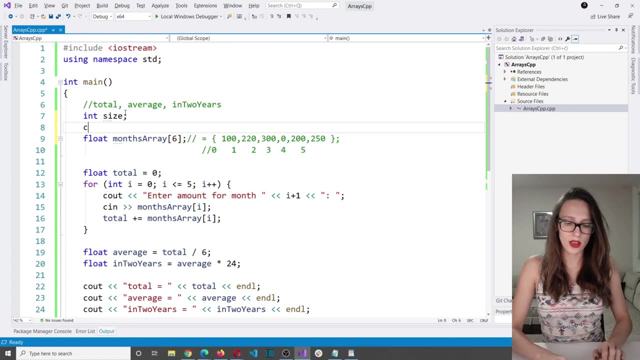 Wouldn't it be super interesting to have a set of indexes from zero to five? Wouldn't it be super extra cool if we could do something like this? So we create a variable, we call it size, and then we ask our user to enter the value for that variable. And what do we do with this? 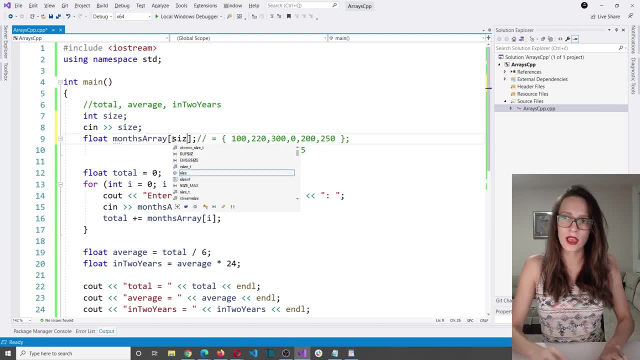 variable. Well, we put it here. So we say that we want to create an array that has this many elements, So the value that our user has entered. So can we do this in C++? What do you think? 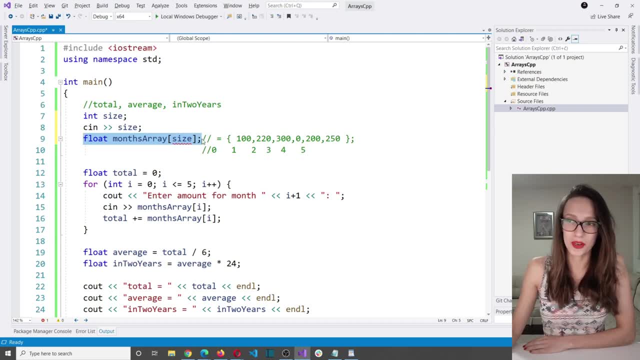 Can we? The answer to that question is no. Unfortunately you cannot do this in C++, but stay with me until the end of the video because I might have a solution for this. So the error that we get here says it says expression must have a constant value. 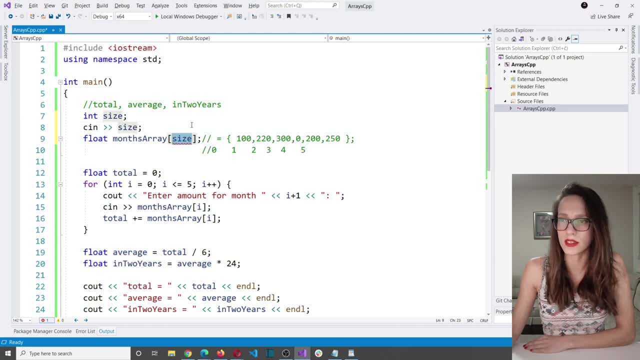 which means that this value here has to be a constant. Basically, it has to be known before you compile your program or before you run your program. So this value here has to be hard coded. Now I want to explain some characteristics that are related to Array. 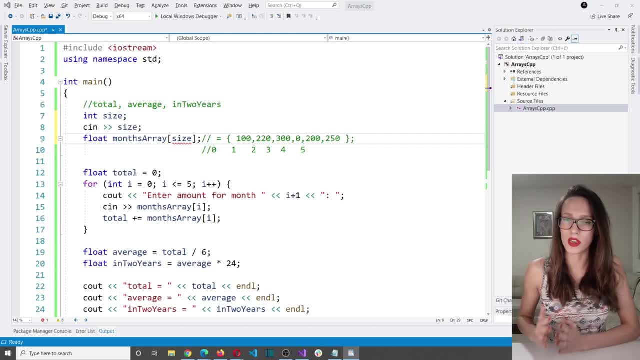 that I haven't mentioned before and you need to be familiar with those characteristics in order to really understand arrays. So an array is type of collection which stores data in continuous chunk of memory. So that means that once you create that array, 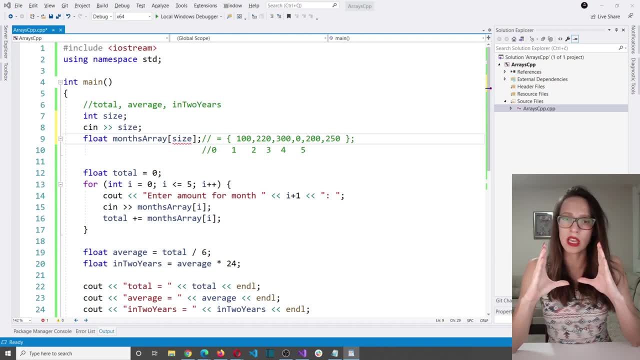 array takes a continuous chunk of memory in your memory and it stores all of the elements, one after the other, in that chunk of memory. Now that means that you cannot add more elements to that array. So you cannot add an element at the end, in the middle, in the beginning. You cannot. 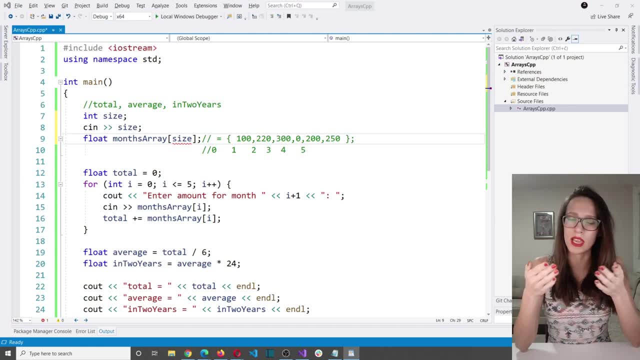 do that, And if you need to add more elements to your array, the only way to do that is to create a bigger array and then to copy that smaller array, And you will still have a remaining space for the new values that you want to store in your array. So that is the only way to have more. 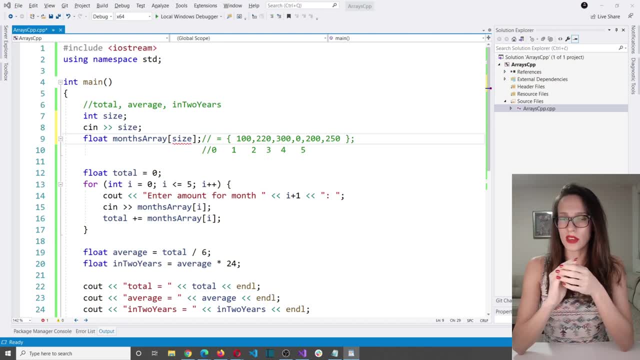 elements added to your array. So that is one obvious disadvantage of arrays. But the fact that arrays store elements in continuous memory has certain advantages as well, And the main one is that accessing and finding elements of arrays is very, very fast. Why? Well, because if you want to, 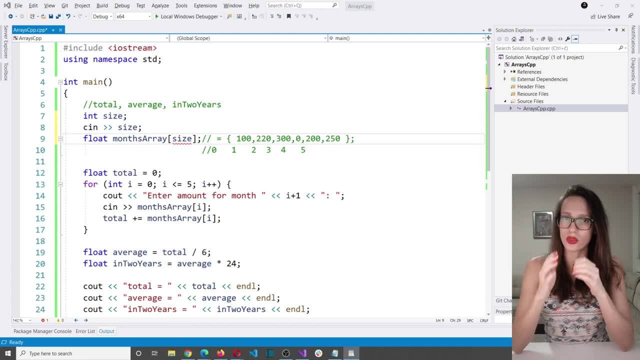 for example, find the element of the array that has index 2, you know that you will have to look only in this fixed chunk of memory And the element that has index 2 is probably going to be somewhere in the beginning of that array, Whereas if you use some other data collection which stores data in non-continuous 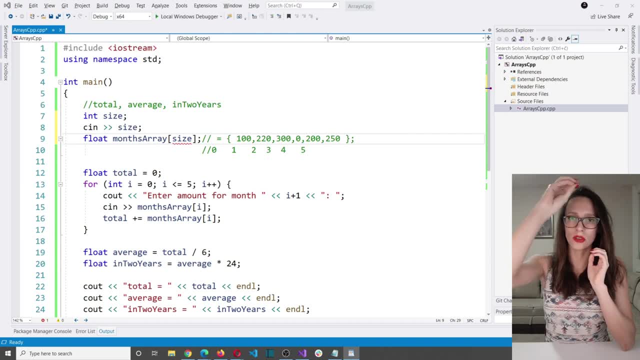 memory, which means randomly all around your memory. accessing and finding elements in that collection is going to be much, much slower. And one example if you have a data collection that stores data in non-continuous memory is linked list. But we will be talking about linked lists. 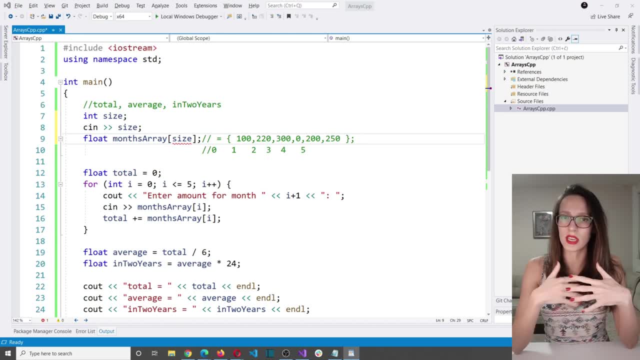 in my future videos. So I will make a separate video which is going to be dedicated only to linked lists. But again I want to say that arrays and linked lists as well have certain advantages and disadvantages. So in arrays, more specifically, it is that accessing elements of the